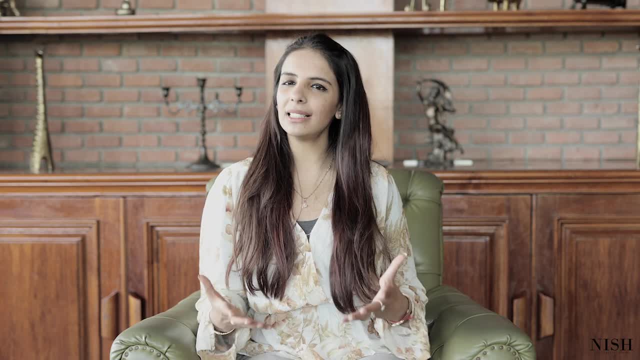 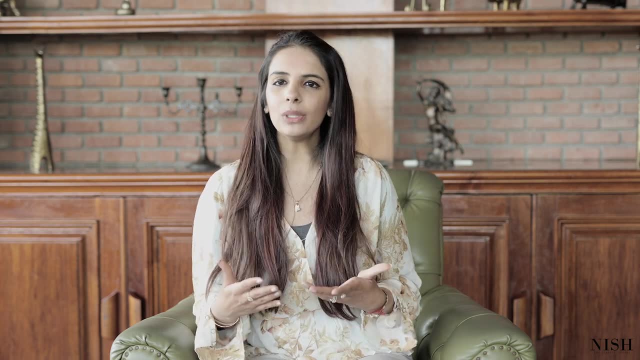 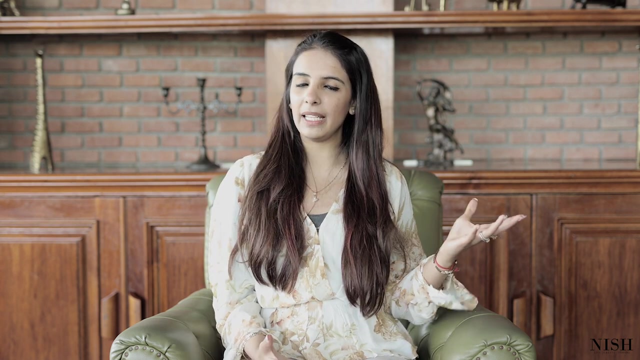 Well, to start with the grey paint colours, you must know that there is no generic grey paint colour. When diving deeper into the category, you would see that some grey paint colours are very neutral and have a very little touch of warmth, whereas some grey paint colours, as I call them, warm grey. 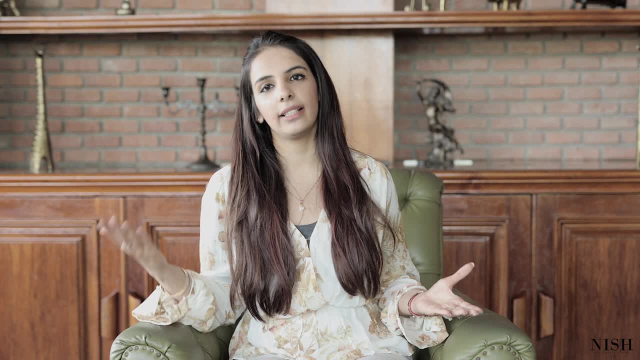 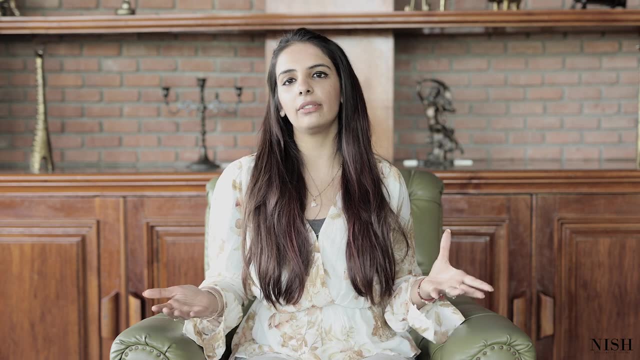 are greige paint colours and some are icy, cool grey paint colours, And I know that it can be quite overwhelming for you, And that is why here is a graphical representation of all these three paint colours. The grey paint colours can further be sub-categorised. 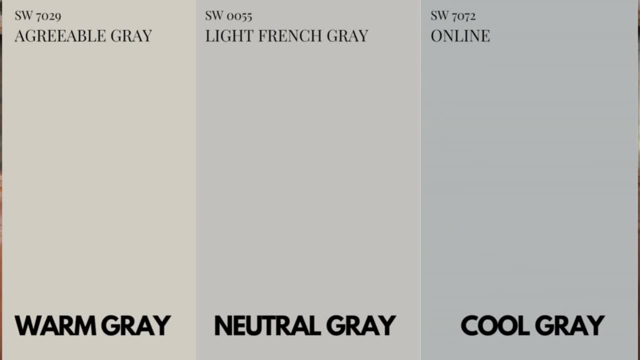 into warm grey, neutral grey and cool grey paint colours. Sherwin-Williams Agreeable Grey is a warm grey paint colour. Sherwin-Williams light French grey is a medium toned neutral paint colour that is neither very warm nor very cool, and Sherwin-Williams online is a perfect. 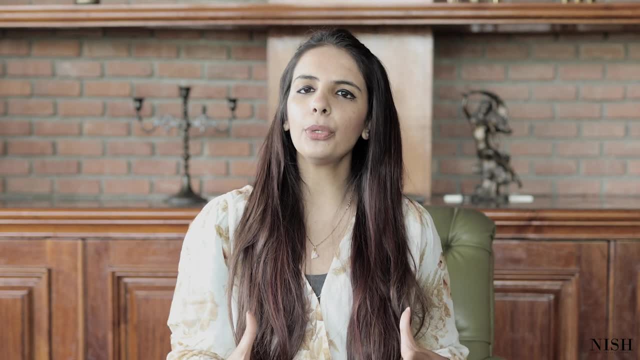 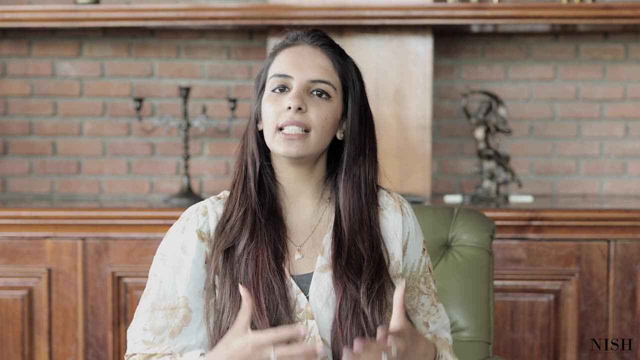 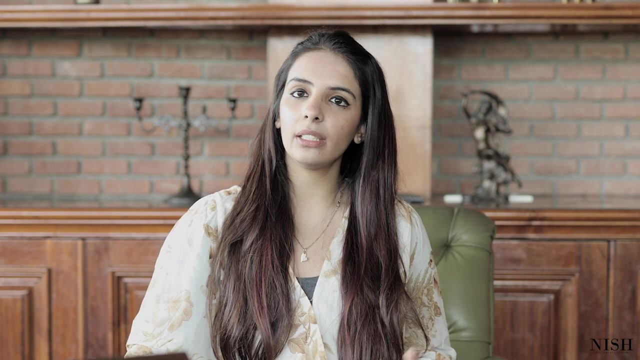 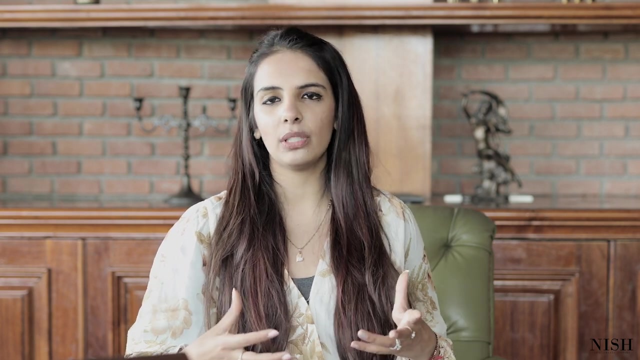 example of a cool toned grey paint colour. Now, how would you know which particular grey paint colour is best suited for your space? Well, keep in mind the existing architectural elements: the natural stone, the wooden countertops, the wooden flooring and several other complementary colours of your home. So if you have majorly warmer tones running around your house with 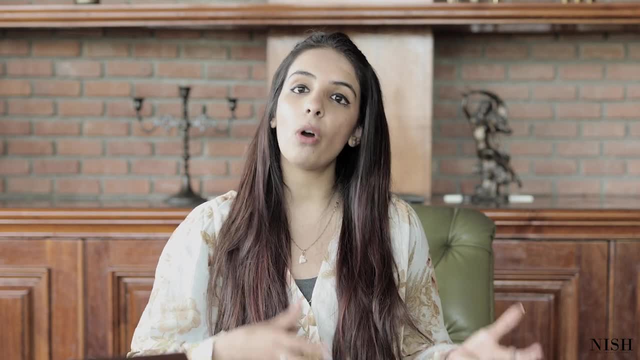 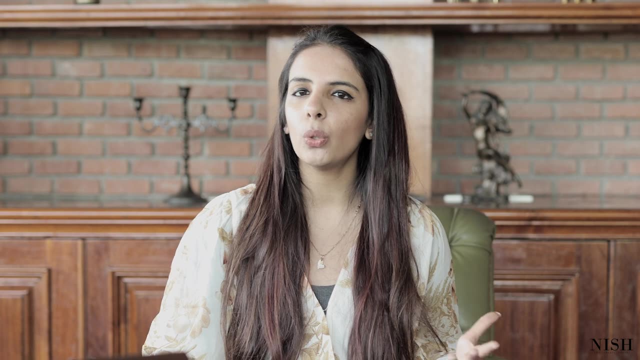 ample wooden textures, it's ideal that you choose a warm grey or neutral grey paint colour. On the other hand, if you have cool toned natural stone, cool toned colour palettes, ample whites and blacks, then it's ideal to choose a cool toned grey. especially if it's a coastal shabby chic or even a contemporary or Scandinavian interior design style, Don't make a mess and paint it. vice versa, If you have warmer tones running around your house and you love the feel of greys, it's ideal that you choose a warm grey paint colour as opposed. 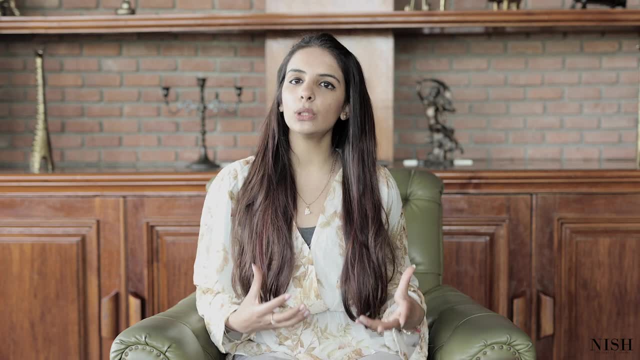 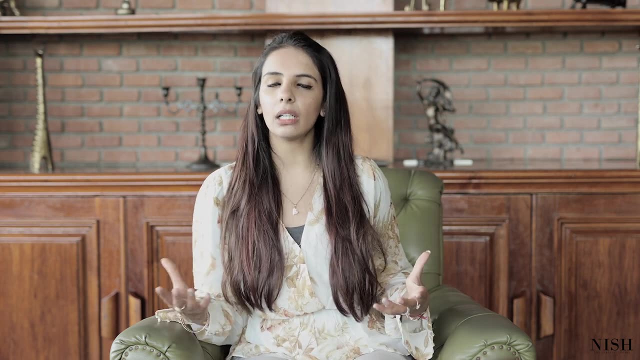 to cool grey paint colour. These grey paint colours can also be further sub-categorised based on their light reflectance values- How light, medium or dark a paint colour can be, And this solely depends on the size of your space. So if you have larger spaces, 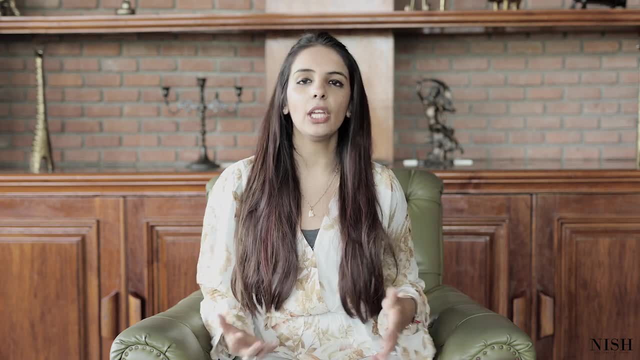 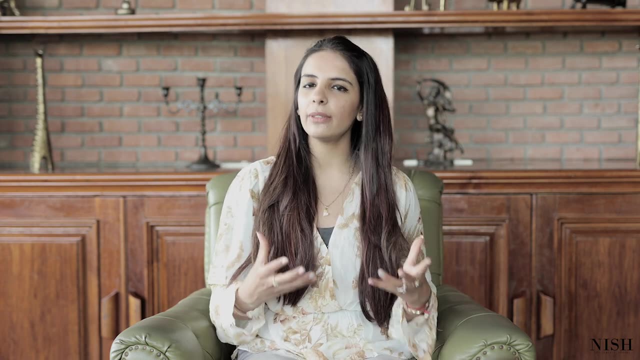 with sufficient natural light entering at all times, you can actually experiment with medium to medium darker grey paint colours. On the other hand, if you're really fond of the grey paint colours and you have a smaller space with very restricted natural light entering, it's ideal. 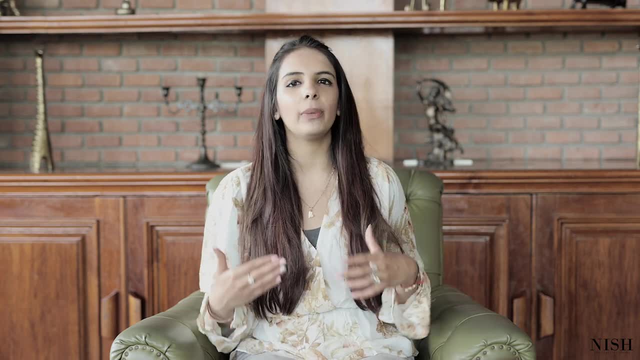 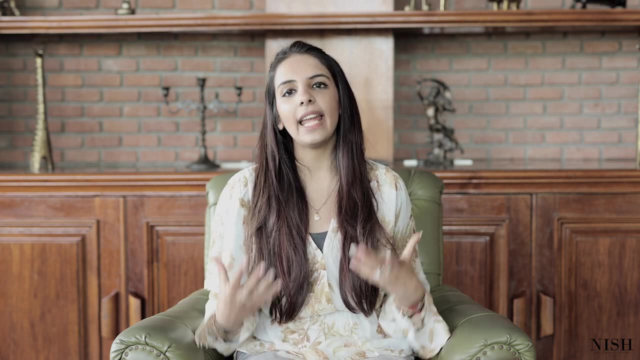 that you choose an off-white with grey undertones or probably a very lighter tone of grey or even a lighter grey paint colour. Generally, cooler toned paint colours tend to make your space feel much lively and airy and brighter. So if you're looking to make your space look, 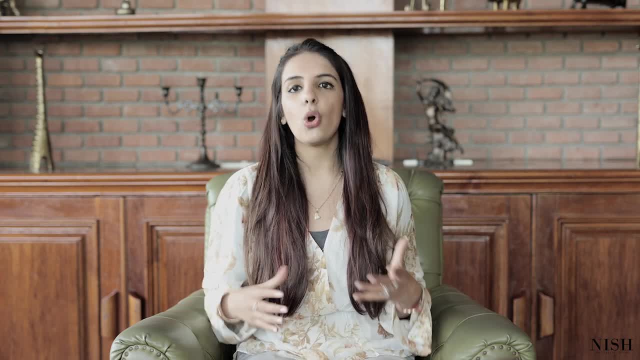 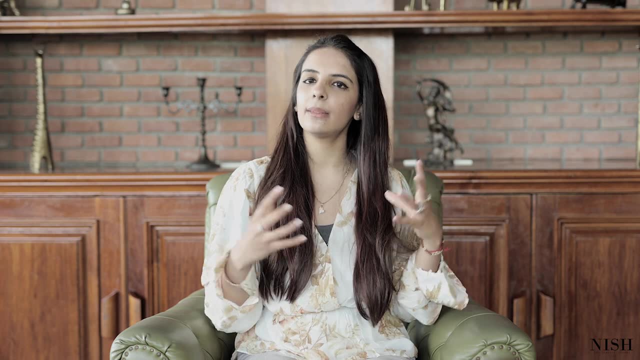 much larger than it already is. lighter greys or cooler greys is your solution. On the other hand, if you're looking to make your space look slightly confined and smaller, then you must choose warmer greys or darker greys. Generally, Sherwin-Williams neutral grey paint colours are the best to go. 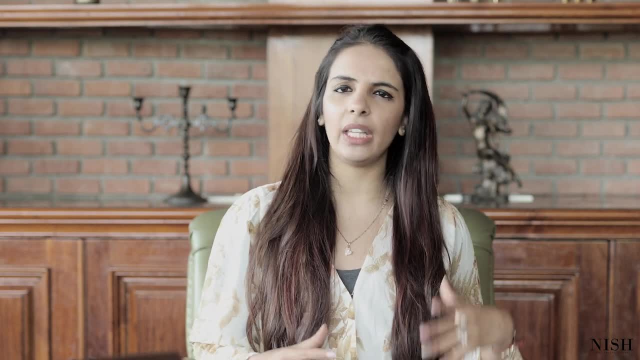 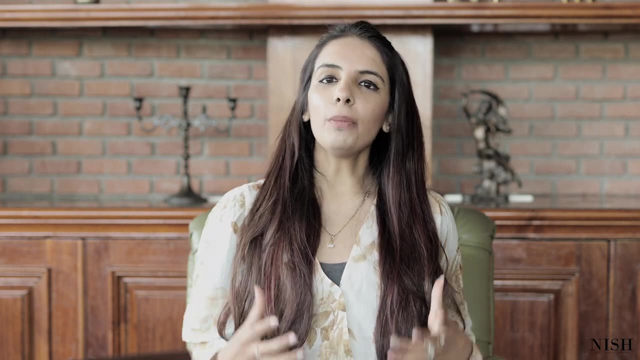 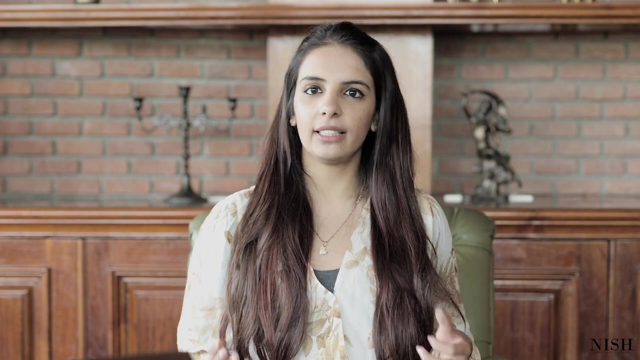 They don't have any undertones, they can easily blend with any existing architectural elements, any existing colours or materials, and will never disappoint you. So to make it easier for you, here's a quick roundup of the best grey paint colours, based in each categories. 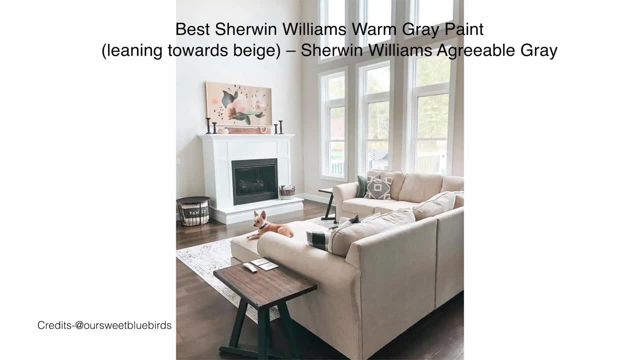 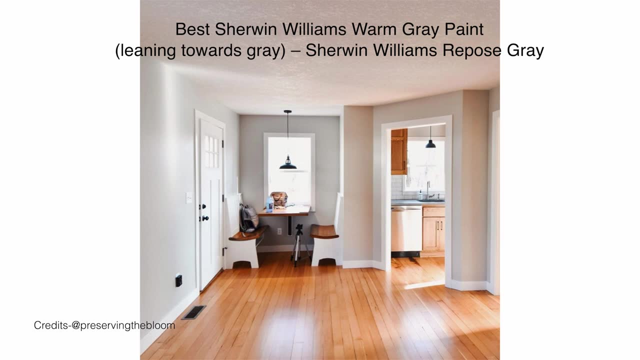 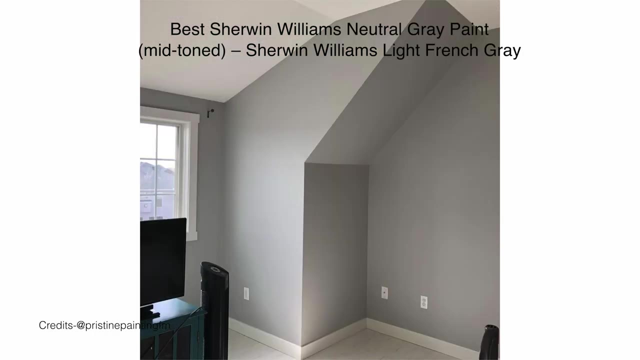 Let's get started. The best Sherwin-Williams warm grey paint colour that leans towards beige is Sherwin-Williams Agreeable Grey. The best Sherwin-Williams warm grey paint that leans towards grey is Sherwin-Williams Repose Grey. Best Sherwin-Williams Neutral Grey paint which is even medium toned is Sherwin-Williams Light. 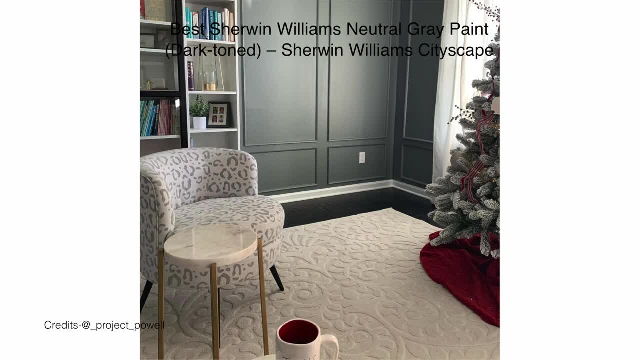 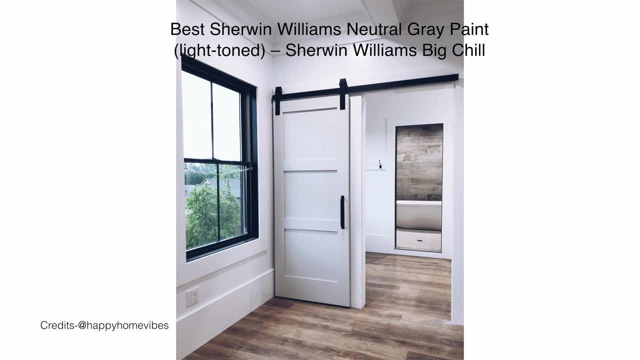 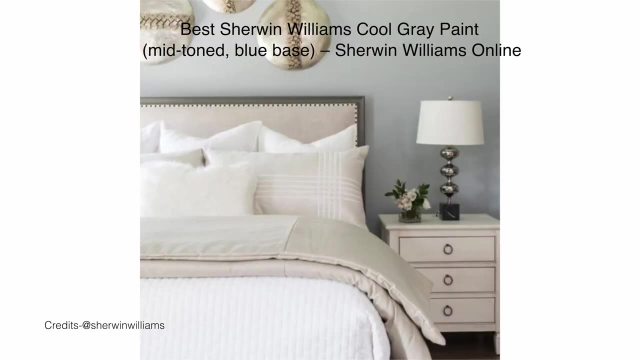 French Grey. Best Sherwin-Williams Neutral Grey paint which is darker toned is Sherwin-Williams Cityscape. Best Sherwin-Williams Neutral Grey paint colour which is lighter toned is Sherwin-Williams Big Chill Best Sherwin-Williams Cool Grey paint, which is medium toned with a blue undertone, is Sherwin-Williams. 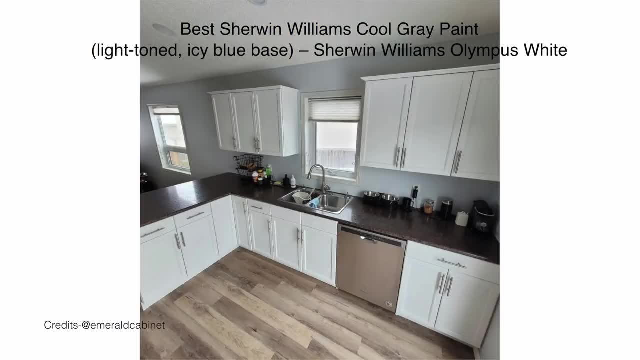 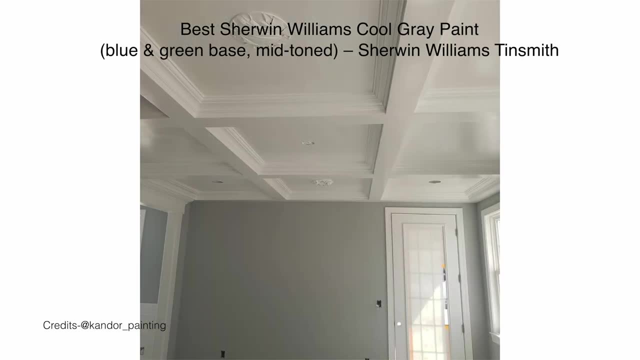 Online. Best Sherwin-Williams Cool Grey paint, which is light toned and has an icy blue base, is Sherwin-Williams Olympus White. Best Sherwin-Williams Cool Grey paint, which has a blue green base and is a medium toned colour, is Sherwin-Williams Tinsmith. 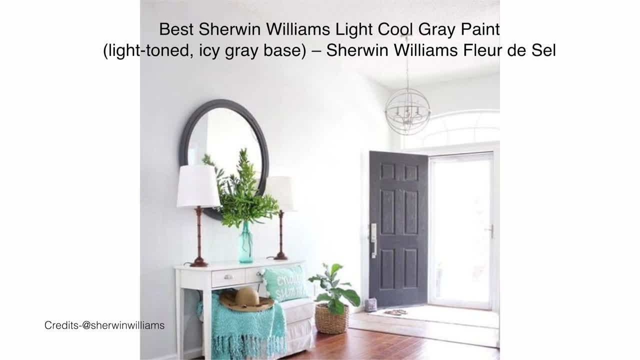 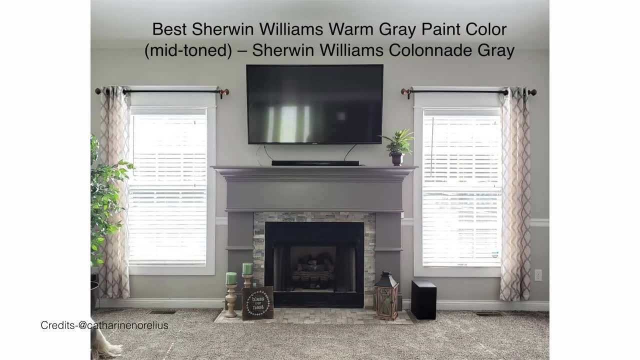 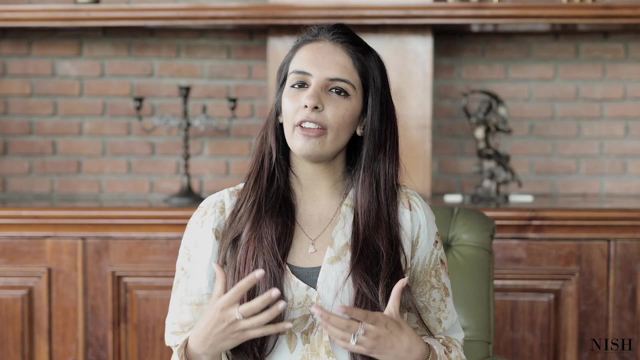 Best Sherwin-Williams Light Cool Grey paint, which is light toned and has a blue undertone, a very light, icy grey base, is Sherwin-Williams Fleur de Sel. And lastly, best Sherwin-Williams warm grey paint colour which is medium toned is Sherwin-Williams Colonnade Grey. So now that I've 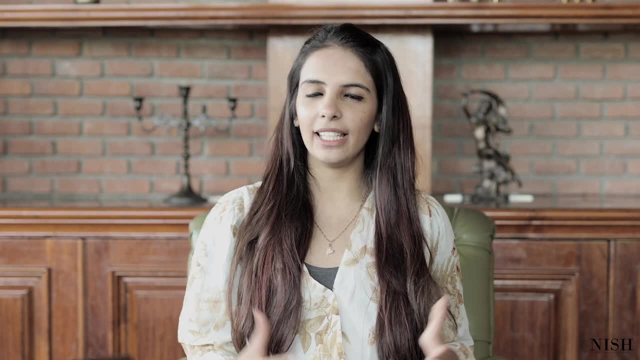 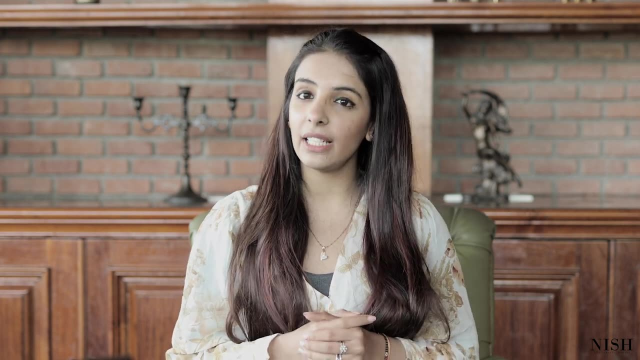 briefed out the best paint colour for each category. let's get started with my top 10 picks of Sherwin-Williams grey paint colours that you can definitely have an eye on. You can use these paint colour in your home, and I'm going to share my thoughts on each and every one of those. 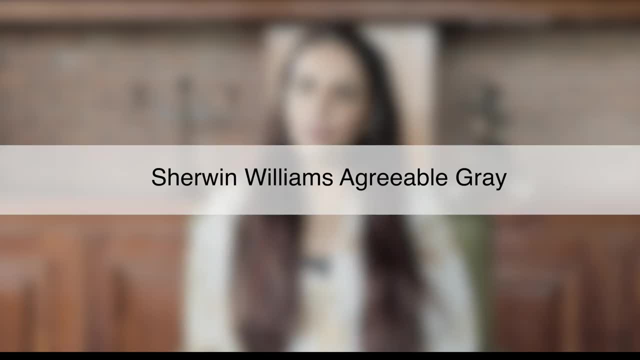 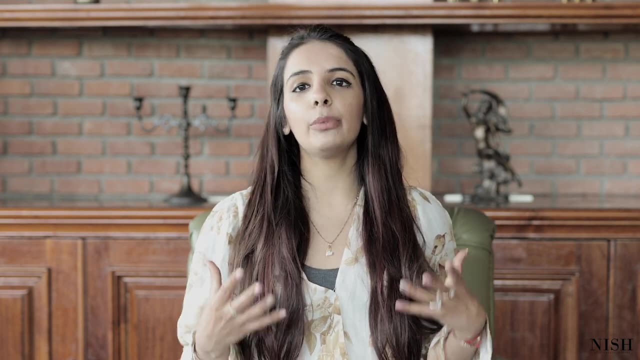 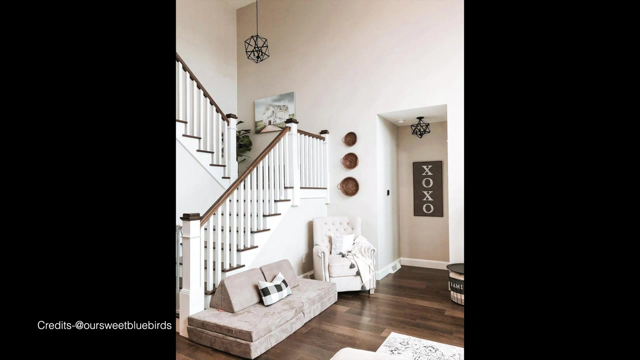 colours. Let's get started. Sherwin-Williams Agreeable Grey. Well, Sherwin-Williams Agreeable Grey is an effortless, warm grey paint colour with deep taupe undertones. It's a versatile, warm grey paint colour that is quite likely to make your space feel calm and subtle, This grey paint colour. 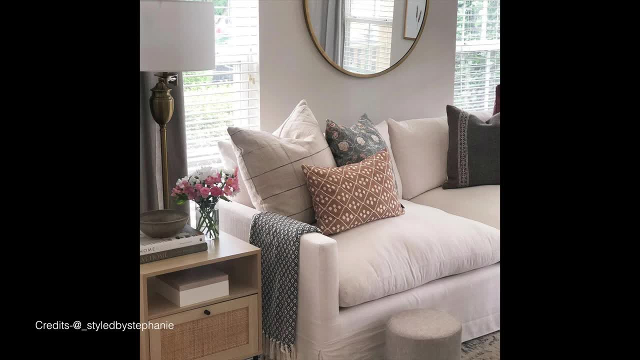 definitely falls on the warmer end of the scale, hence not too warm. So if you compare it with Sherwin-Williams Agreeable Grey, it's a very warm grey paint colour. It's a very warm grey paint colour. If you compare it with Sherwin-Williams Accessible Beige, you would see that this grey 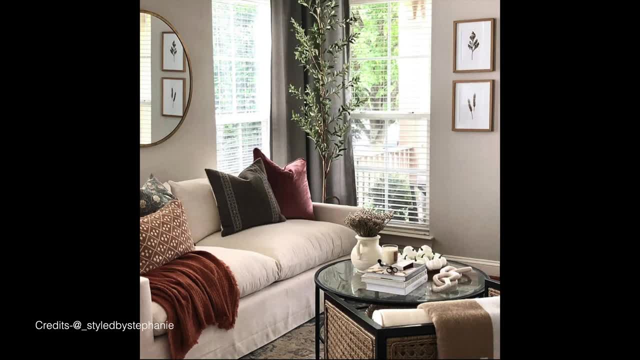 paint colour definitely has a deep grey undertone. If you're looking for a paint colour slightly warmer than Sherwin-Williams Agreeable Grey, then choose Sherwin-Williams Accessible Beige. So if you're looking for a paint colour which is slightly warmer than Sherwin-Williams Agreeable 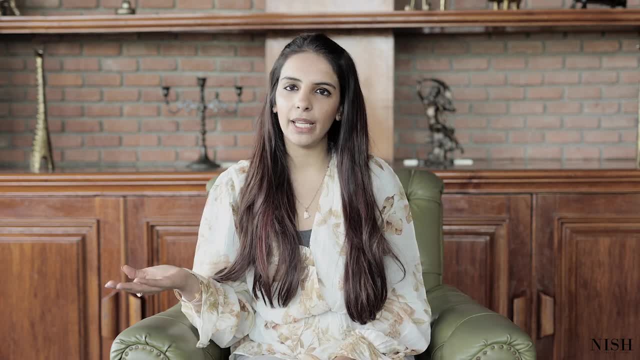 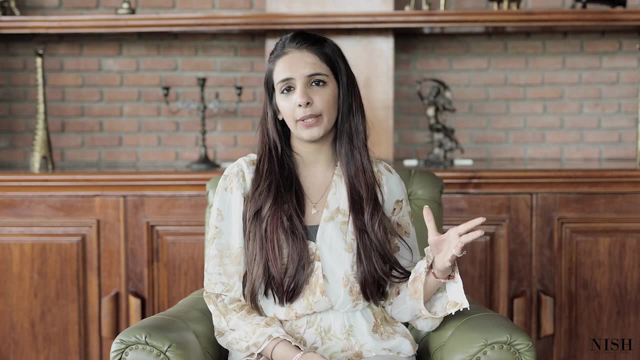 Grey, then you must choose Sherwin-Williams Accessible Beige. On the other hand, if you're looking for a slightly cooler toned colour as compared to Sherwin-Williams Agreeable Grey, then you must pick Sherwin-Williams Repose Grey for the best results. 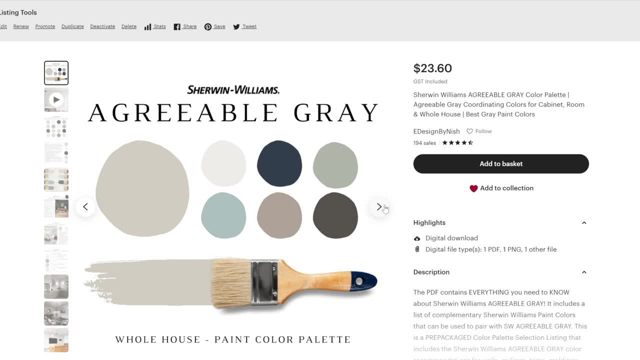 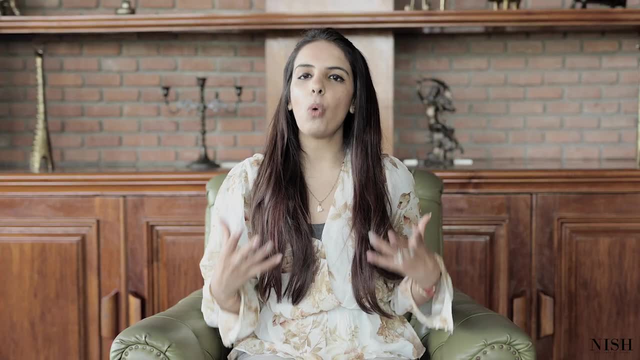 Now here's where you can check out my latest pre-packaged Sherwin-Williams Agreeable Grey colour palette for your whole house. You can find it on Etsy as well as my website. The next wonderful Sherwin-Williams Grey paint colour is Sherwin-Williams Repose Grey. 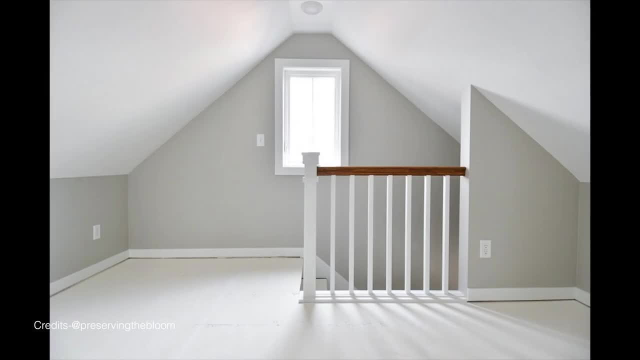 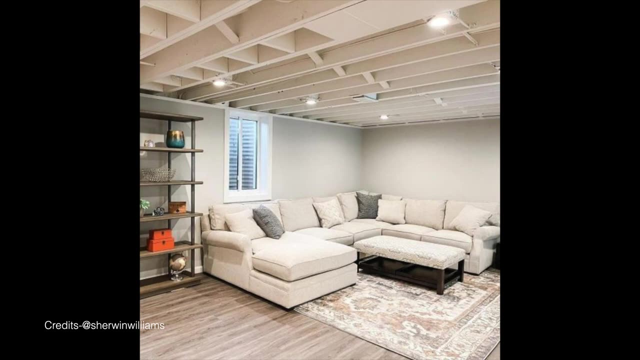 Sherwin-Williams Repose Grey is one grey paint colour with deep brown and taupe undertones. It doesn't feel as warm as Sherwin-Williams Repose Grey, but it's a very warm grey colour. It's not as cool as Sherwin-Williams Agreeable Grey, nor as cool as Sherwin-Williams Passive. 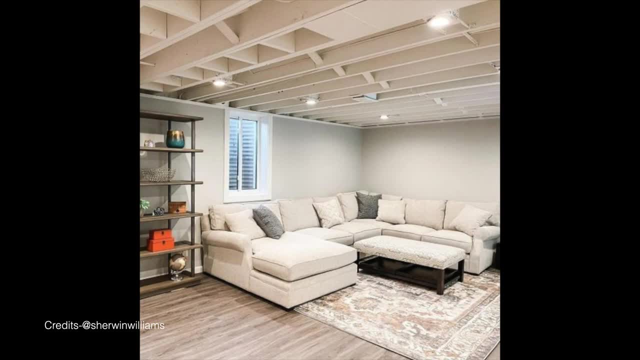 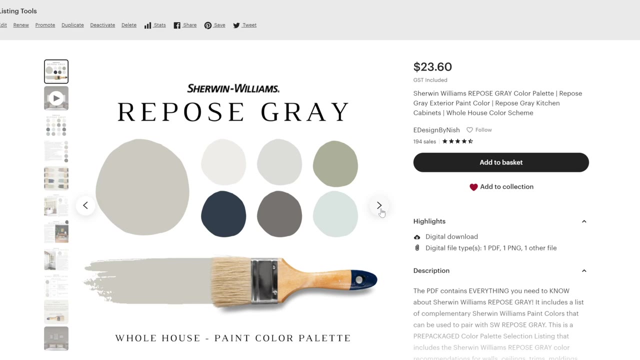 This colour has an LRV of 58 and is falling on the lighter to medium lighter end of the scale. This colour has dominant grey undertones with just a very little touch of warmth to it. Check out my latest pre-packaged Sherwin-Williams Repose Grey colour palette for the whole house. 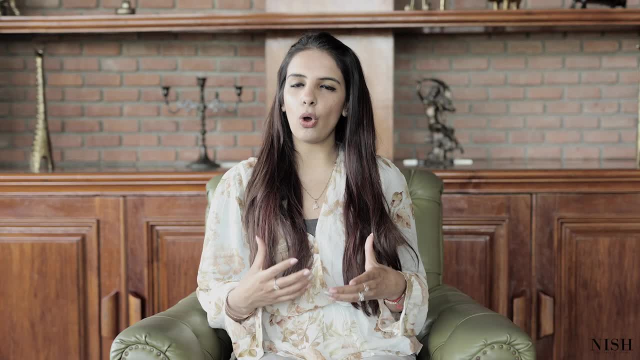 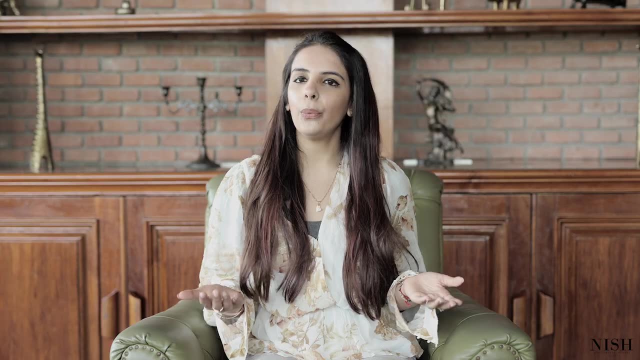 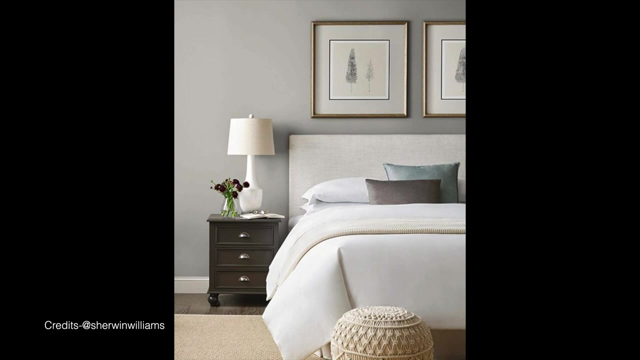 here on Etsy, as well as my website. So now that we have talked about two warm grey paint colours, let's get started with the neutral toned grey paint colour. Well, yes, Sherwin-Williams Light French Grey. Sherwin-Williams Light French Grey is a perfect shade of generic grey. that's neither too cool. 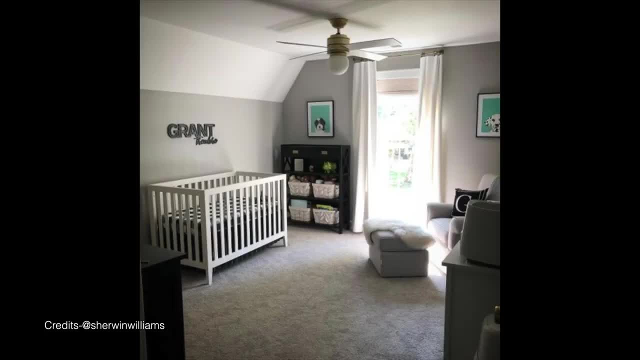 nor too warm. This paint colour can easily blend with any other interior design, style, decor and material. So if you're looking for a grey paint colour that is slightly on the neutral end of the scale, Light French Grey is definitely something to steal an eye off. 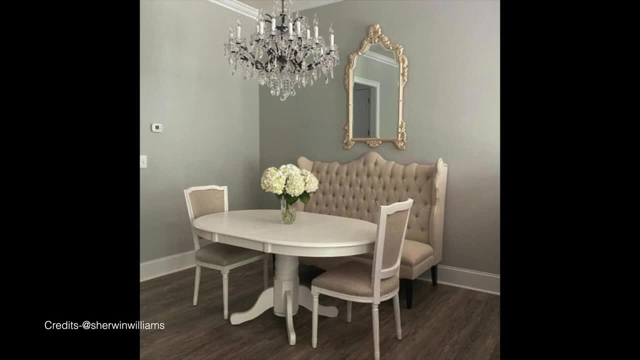 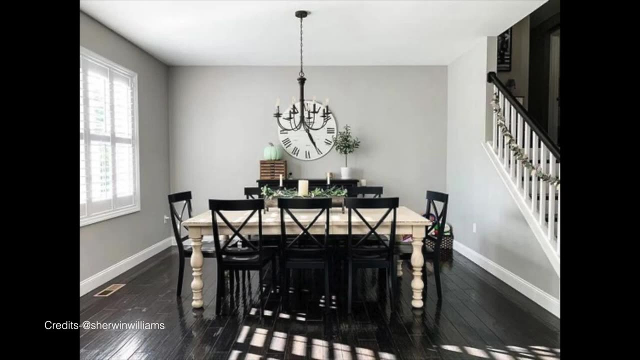 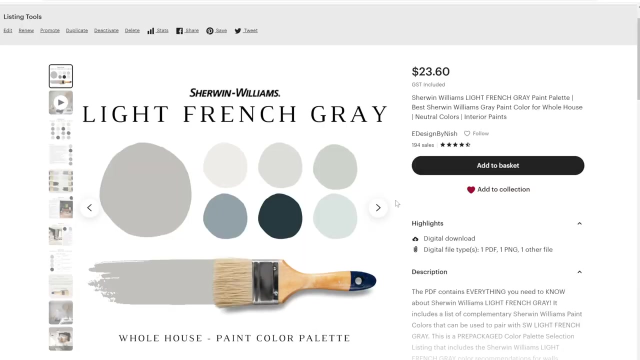 This colour pairs beautifully with fresh white paint. You can even use it as a base colour. If you're looking for a very warm or icy grey paint colour, this is definitely not your answer. You can also check out my latest pre-packaged Sherwin-Williams Light French Grey palette. 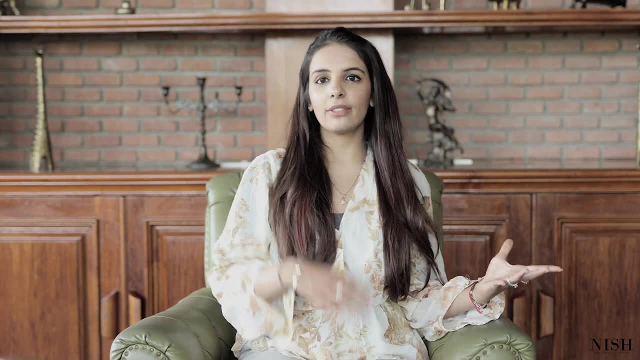 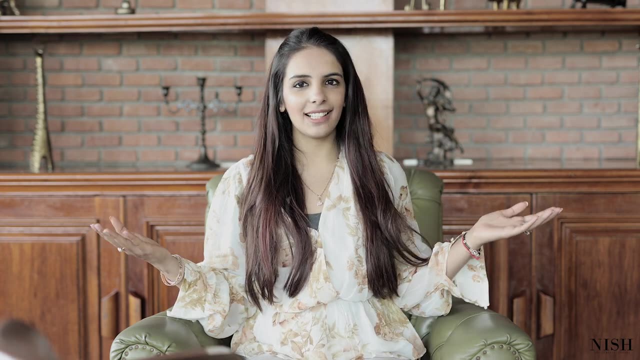 for the whole house here. Now that we've discussed the warm greys, the neutral greys, it's time that we grab attention of the cool grey paint colour. Well, any guesses? Well, yes, Sherwin-Williams online. Thanks for watching. 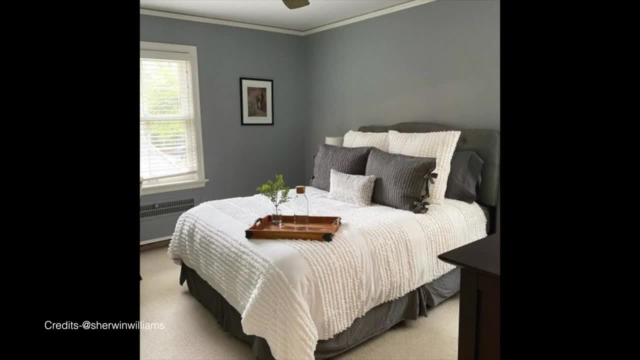 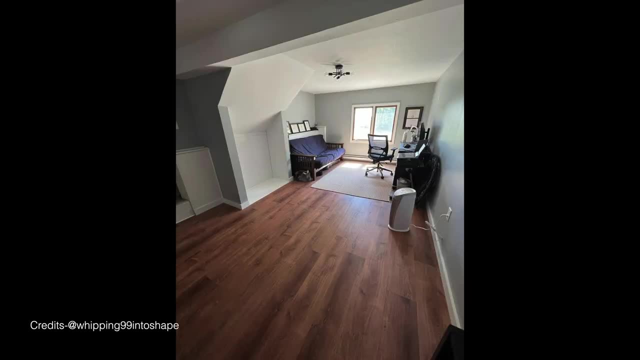 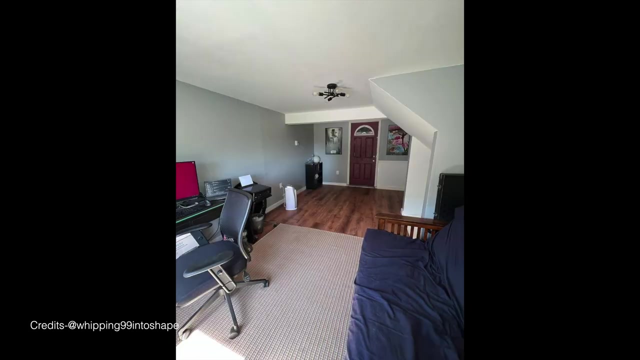 Bye, Bye. Sherwin-Williams online is a pretty cool grey paint colour that can potentially hint at slightly blue undertones. It's cool, calm, crisp and can be termed as a true cool grey paint colour with deep blue undertones. This is a medium tone paint colour so you have to be slightly careful around where you. 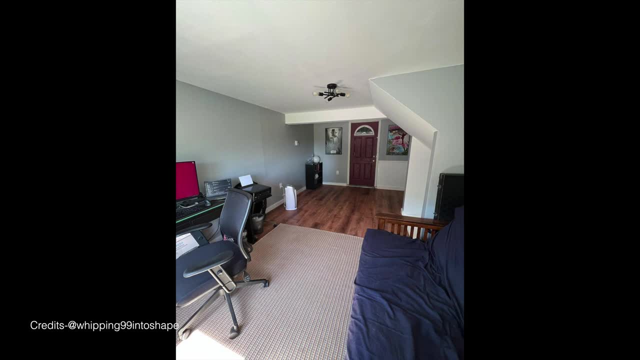 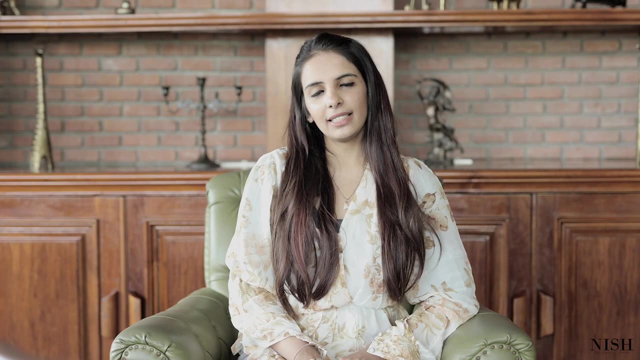 intend to use this paint colour, This cool tone grey has crisp appearance which can appear slightly blue in the north facing rooms and grey in the south facing rooms. So be careful in the south facing room. Next in the line is Sherwin-Williams Big Chill. Sherwin-Williams Big. 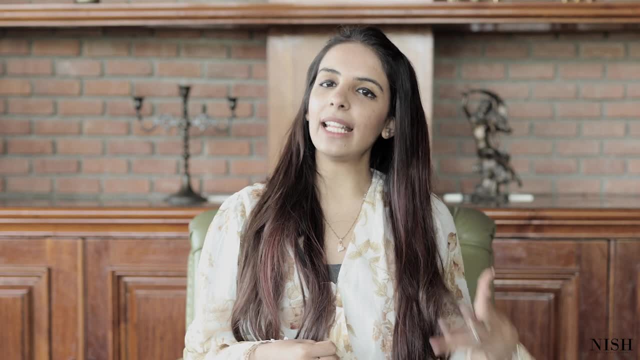 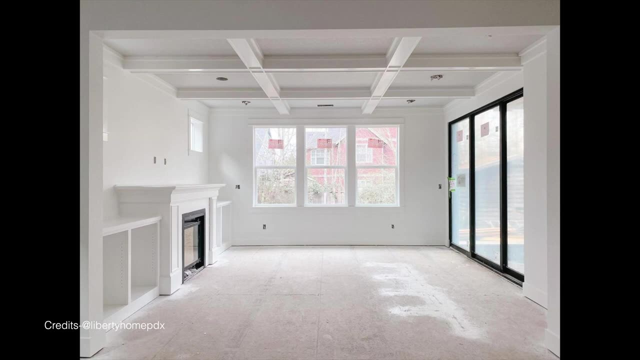 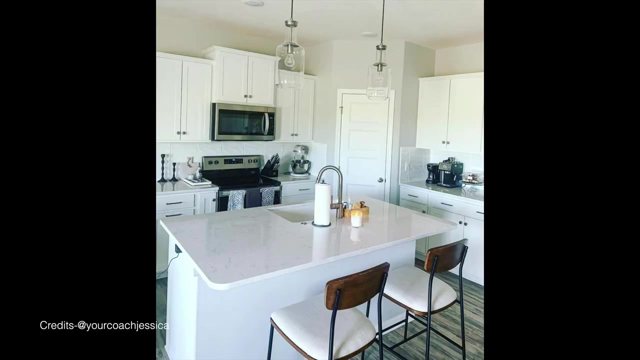 Chill is an icy grey paint colour which is lighter in tone and can hold itself excessively well in brighter rooms. This colour is also an ideal paint colour for darker rooms or rooms receiving little natural light, With a tiny wink of stormy blue undertones which aren't very dominant, this paint 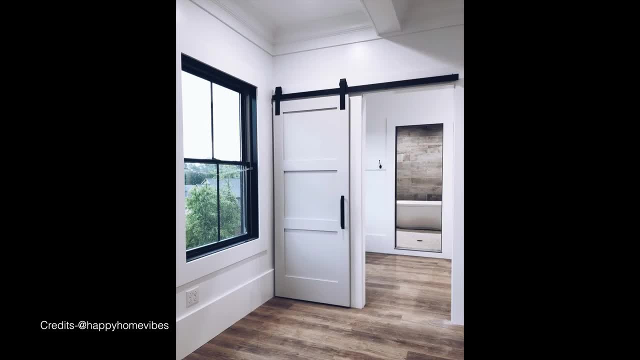 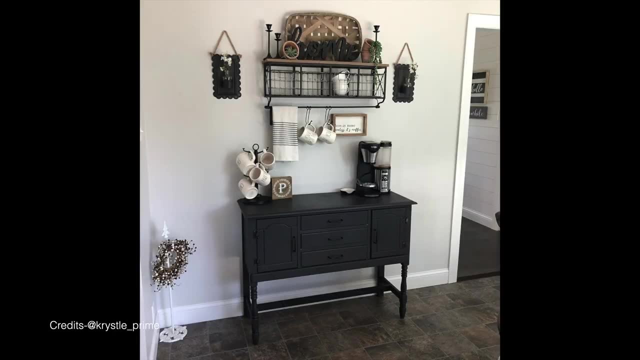 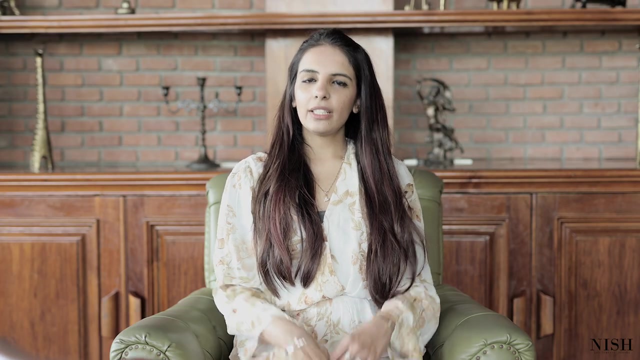 colour is definitely a go-to solution if you're looking for a cool toned light and airy grey paint colour. However, this colour is definitely not very frosty or icy. Sherwin-Williams Big Chill can also be used as a whole house colour scheme. Next in the line is Sherwin-Williams Cityscape. 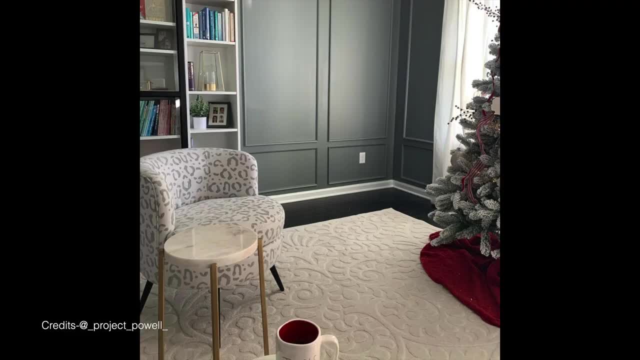 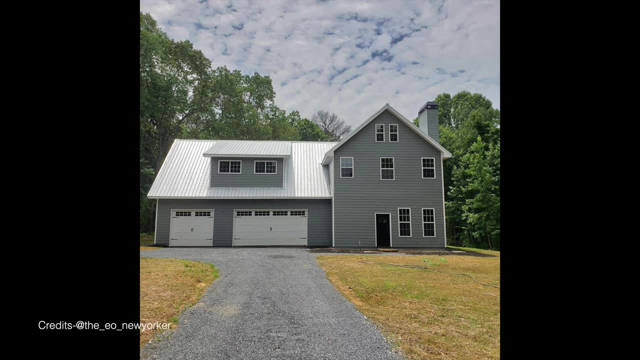 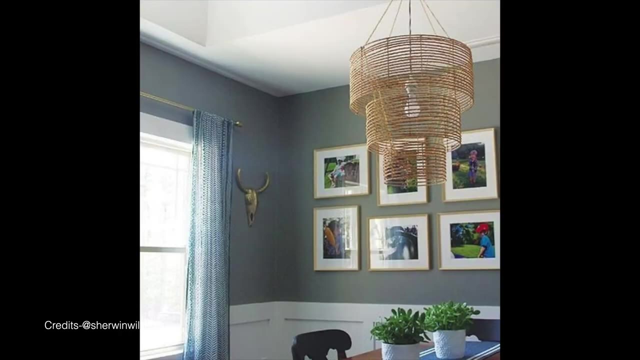 Sherwin-Williams Cityscape is a dark and bold neutral grey paint colour with an LRV of only 22.. This neutral paint colour can be used as an accent in your kitchen, the mudroom, the bathroom, the vanity and the home office. This colour has a very teeny, tiny tinge of blue which is very subdued, hence only visible. in the north facing rooms. The next colour in the line is Sherwin-Williams Olympus White. This colour can be used as a whole house colour scheme, especially for the coastal homes, and it can make your space look extremely light, airy, breezy at all times. 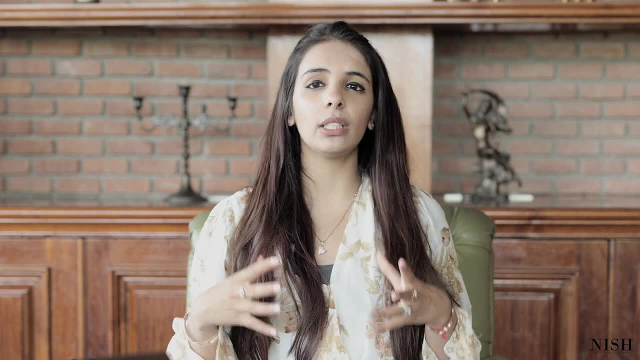 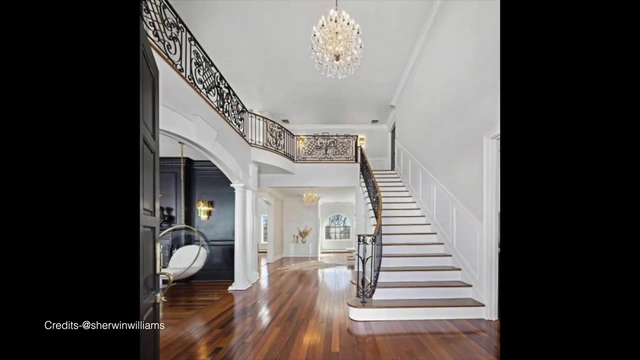 So if you're looking to make your space look much cooler, calmer, crisper and larger, Sherwin-Williams Olympus White is definitely something to have an eye on. However, this refreshing, frosty and crisp colour has a deep touch of blue and grey to it. It pairs beautifully with bold. 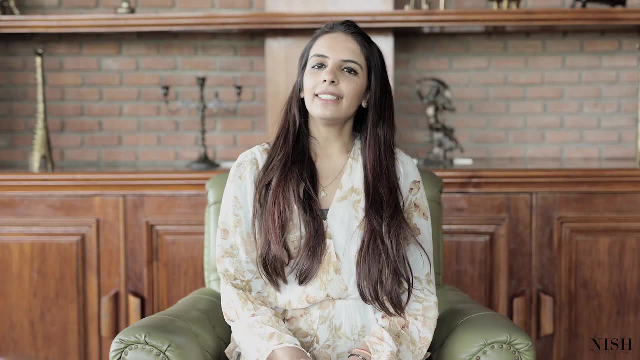 blues, blacks and darker hardwood. The next grey paint colour in the line is Sherwin-Williams Tinsmith. Sherwin-Williams Tinsmith is a cool to work colour. colour. A kick-in: that軍 lights up your room. next grey paint colour in the line is Sherwin-Williams. Tinsmith is a cool to work colour, A kick-in thatưng ushering your room for aiviline Graduationあぁ, to visit this supermarket sojust because this Russell Whitmanbunghe direkt shows how to survive. 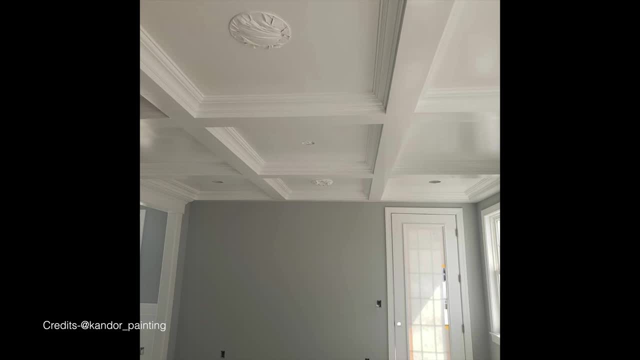 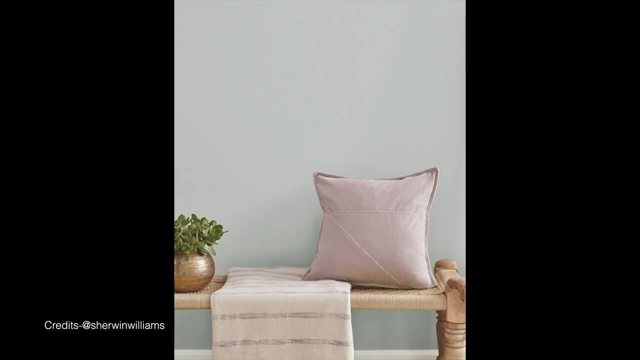 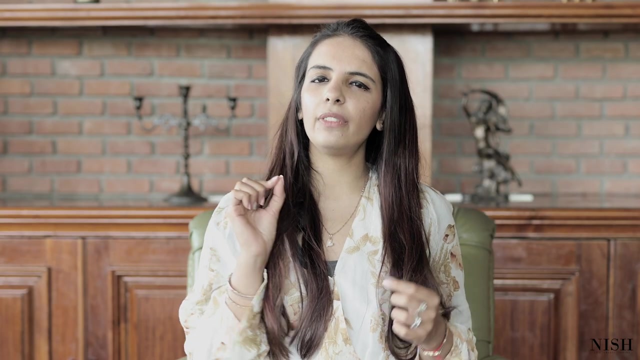 Sherwin-Williams Tinsmith. Sherwin-Williams Tinsmith is a cool tone grey paint colour that isn't icy nor warm. It's a medium toned colour with an LRP of 57 and it can hold itself pretty good in darker rooms as well. The colour has a flash of blue and green undertones to it. 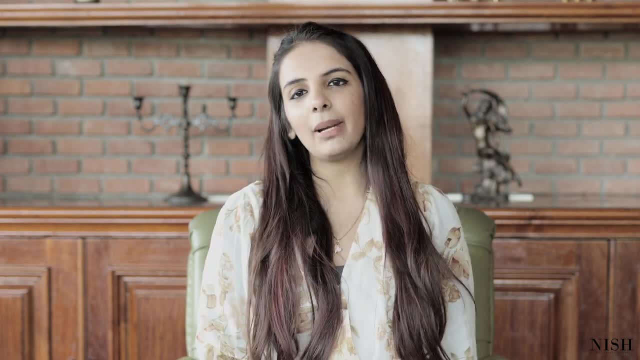 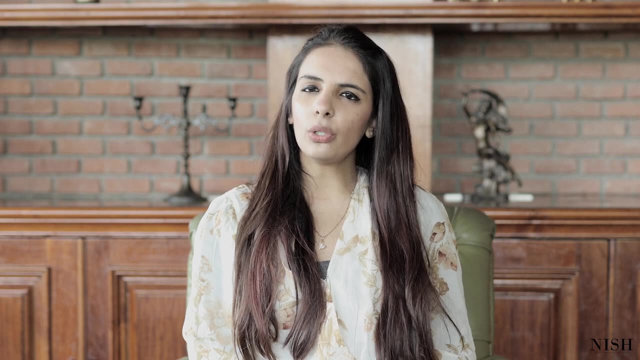 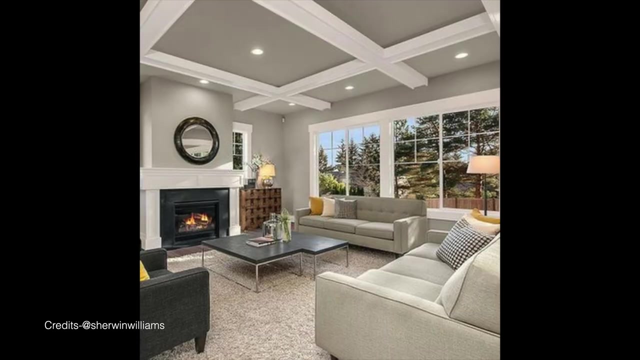 hence you have to be slightly careful what you pair it with. My next top grey paint colour is Sherwin-Williams Colonnade Grey. Sherwin-Williams Colonnade Grey is a stormy, warm grey paint colour with an LRP of 57.. This paint colour falls on the medium end of the scale, is extremely smooth. 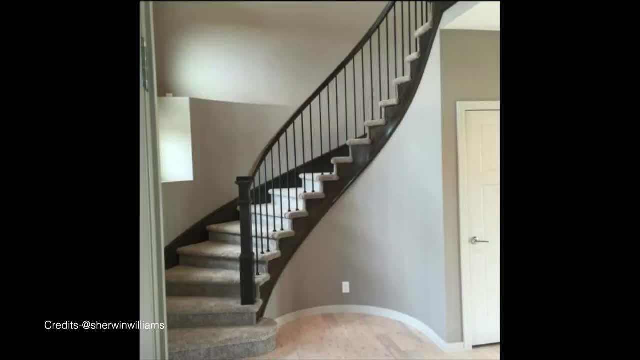 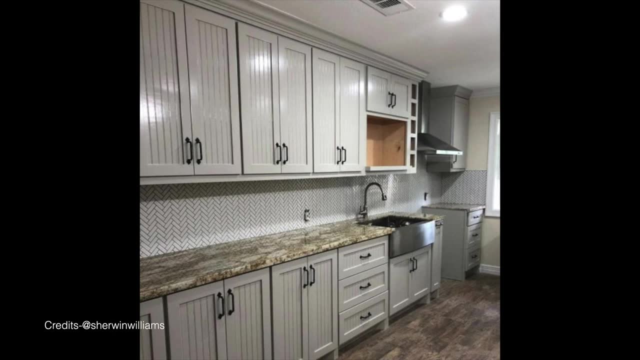 timeless, versatile and can easily blend with any interior design style and decor. However, this paint colour can be a true chameleon. In the north facing rooms it can come off really cool, whereas in the south facing rooms this colour is a true chameleon.